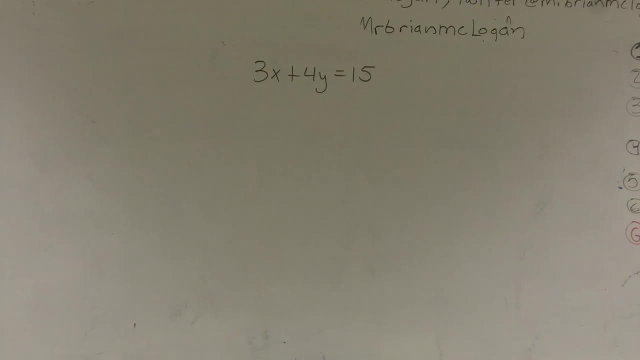 Alright, what I'd like to do is I'd like to show you how to solve a literal equation, solving for x and y. Now, this is very common in graphing, in solving systems, very common in a lot of algebraic techniques. we're going to do, But right now we're just going to practice. 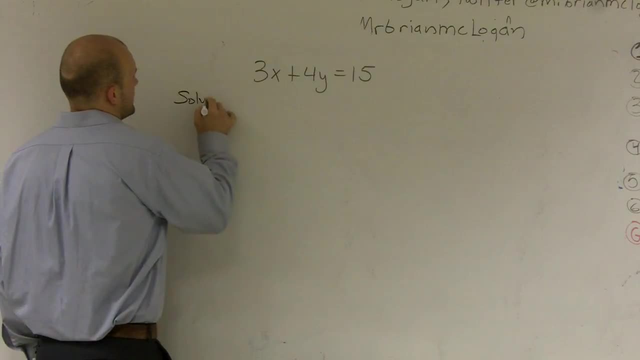 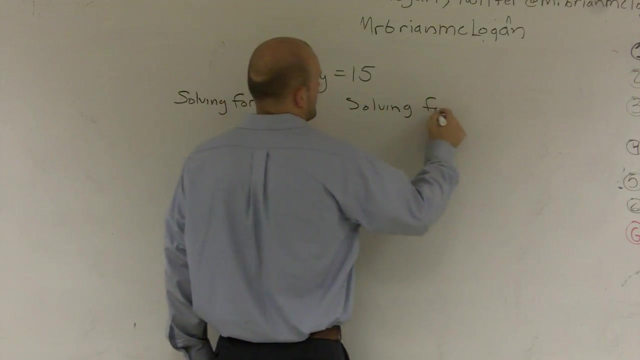 solving for x and solving for y, Alright, so remember, when we're going to solve for x, we want to get x to equal something, and when we solve for y, we want y to equal something. So what I'm going to do is I'm going to show you a couple steps that we can do. First thing, 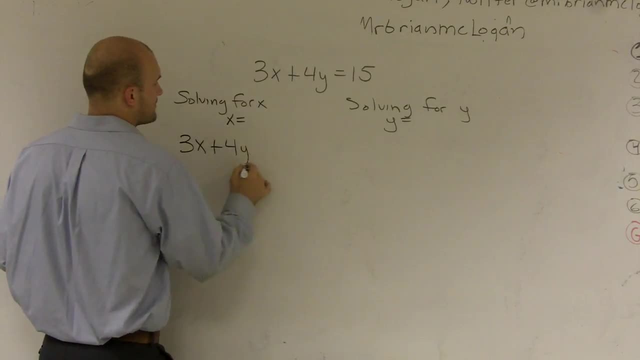 let's just focus on solving for x. If I have, 3x plus 4y equals 15.. Alright, there's a couple operations that we're going to do, So what I'm going to do is I'm going to show you a. 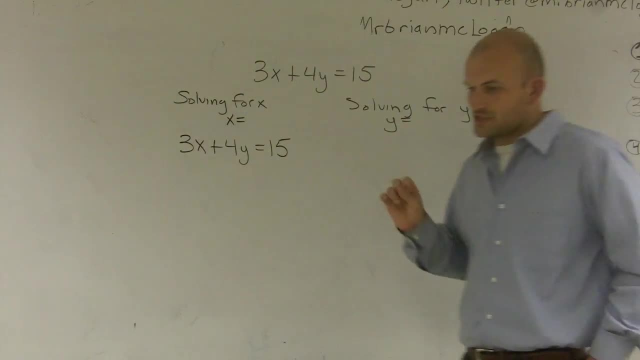 couple operations that we're going to work with right now, And I just want to work on the four operations: adding, subtracting, multiplying, dividing. And for a problem like this, what you guys can see is what are my two operations that are happening? I have 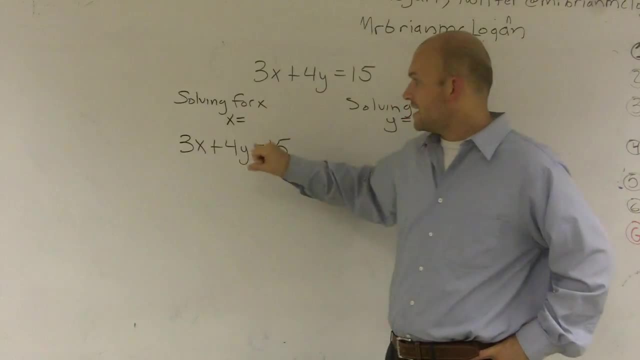 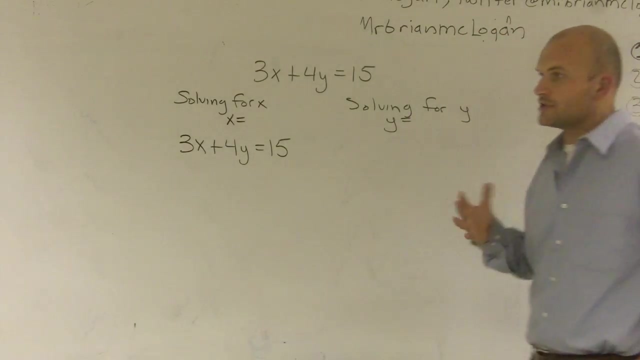 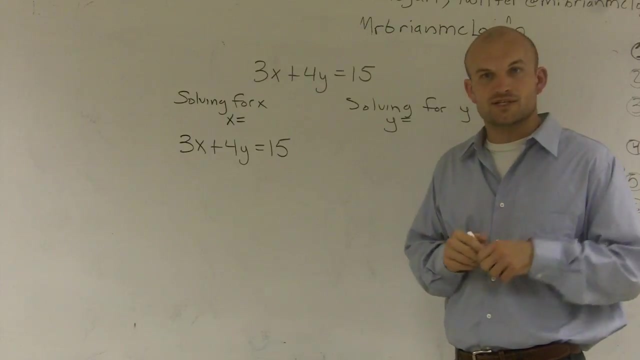 multiplication of my variable times 3, and I have addition of 4y. So when we're solving for a variable, you always want to undo your addition and your subtraction first. So here I'm going to want to undo Addition of a 4y. Well, the undo addition would be subtraction, So I subtract a 4y on. 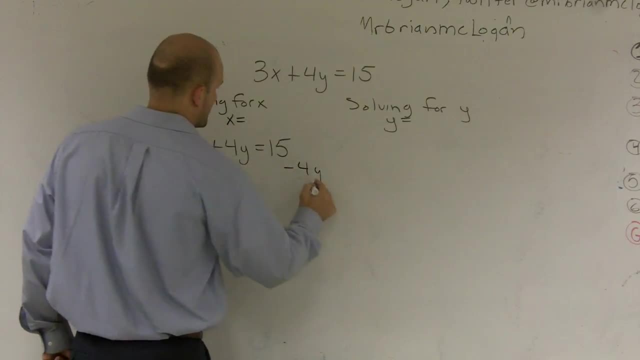 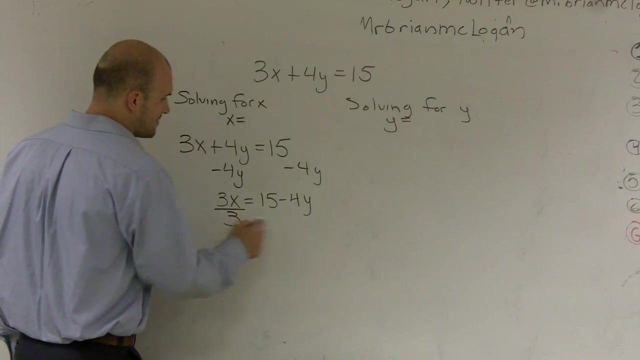 both sides of my equation. Therefore, I get a 3x equals 15 minus 4y. Now I have a multiplication by my variable, multiplication of 3 by my variable. So to do that undo that, I need to divide by 3.. Alright, now remember you cannot combine a 15 minus 4y, So I'm going 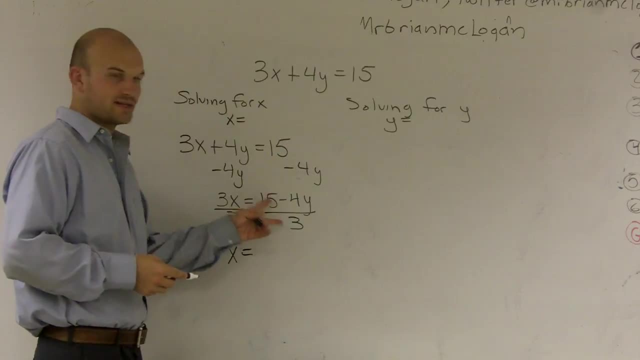 to do that, However, I get x equals, and what I'm going to do is I'm going to separate this into two different fractions: 15 divided by 3 actually reduces down to 5.. And negative 4 divided by 3, I'm just going to keep as a negative 4 thirds y, And that would be my. 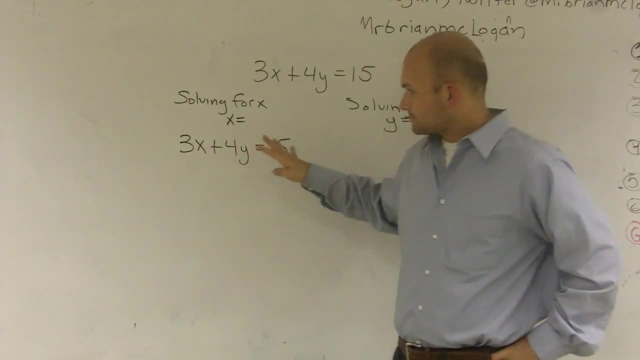 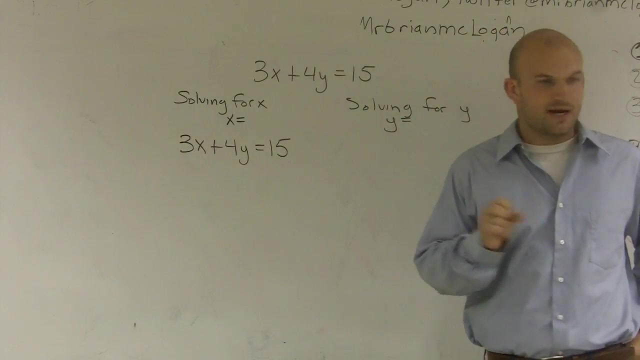 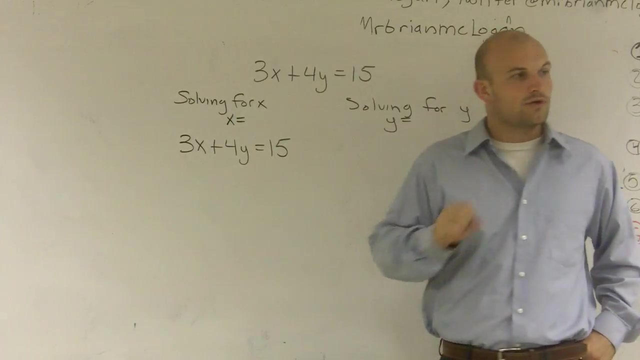 adding, subtracting, multiplying, dividing, And for a problem like this, what you guys can see is what are my two operations that are happening? I have multiplication of my variable times 3, and I have addition of 4y. So when we're solving for a variable, you 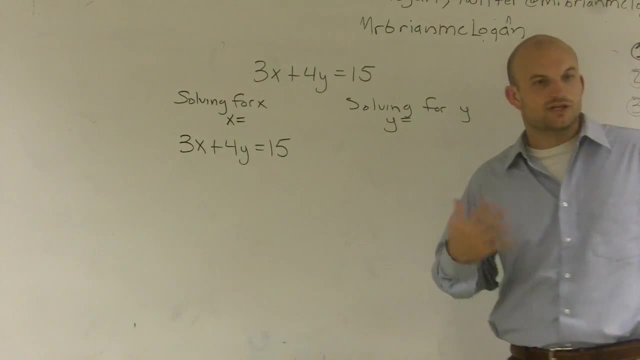 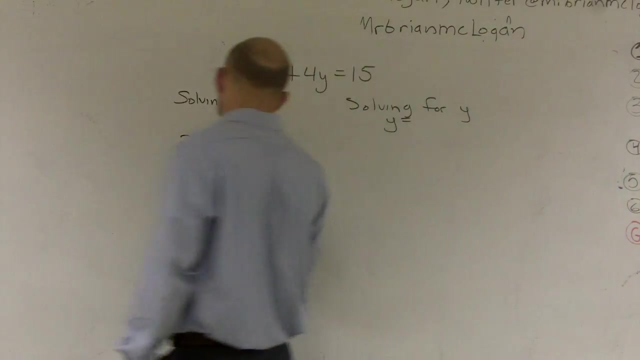 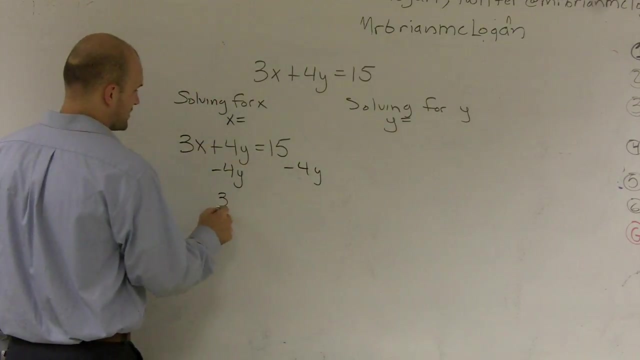 always want to undo your addition and your subtraction first. So here I'm going to want to undo 4y. So what's the undo addition of a 4y? Well, the undo addition would be subtraction. So I subtract a 4y on both sides of my equation. Therefore, I get a 3x equals 15 minus 4y. 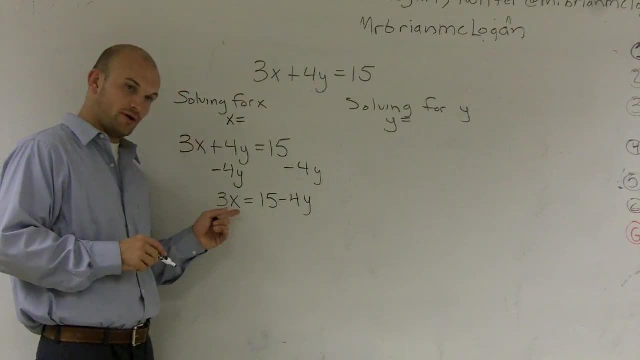 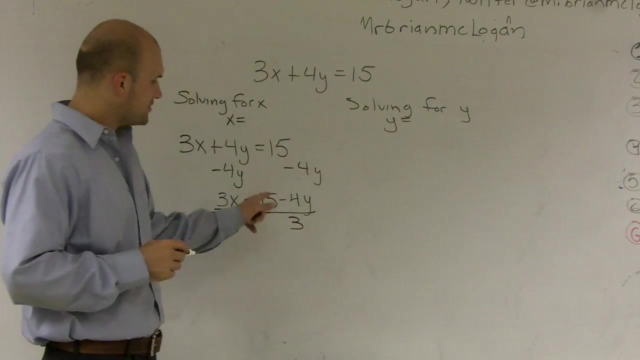 Now I have a multiplication by my variable, multiplication of 3 by my variable. so to do that, undo that, I need to divide by 3.. Alright, now remember you cannot combine a 15 minus 4y. However, I get x equals, and what I'm going to do is I'm going to separate this into 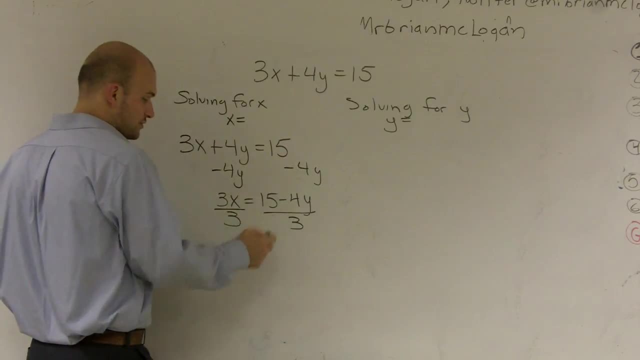 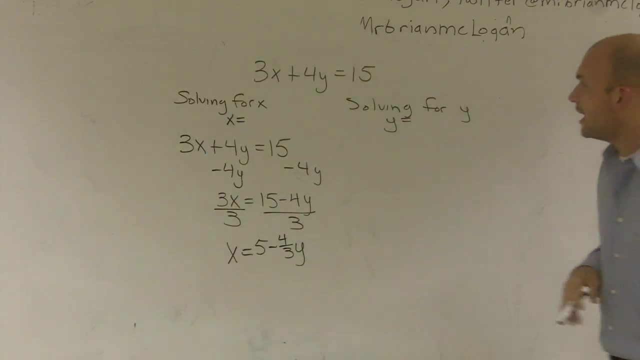 two different fractions: 15 divided by 3 actually reduces down to 5.. And negative 4 divided by 3, I'm just going to keep as a negative 4 thirds y, And that would be my final answer: to solve for x. So now to solve for y. Alright, let's just rewrite it again and see what the 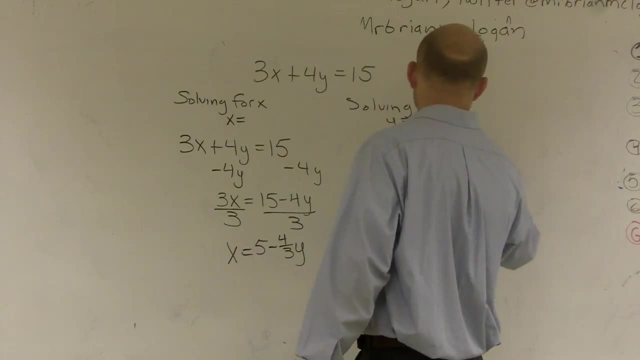 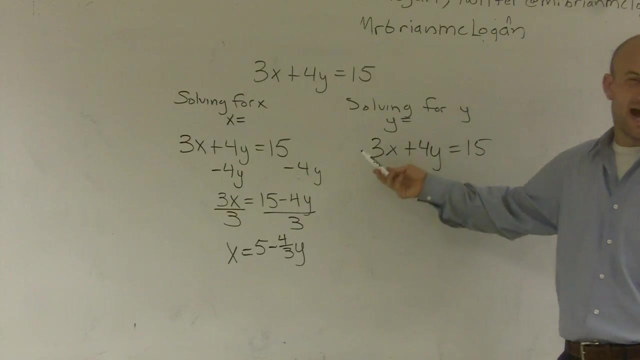 difference is- And there's really actually not too much of a difference because it's both adding. But here again I notice I'm multiplying by 4 and adding by 3x. Alright, this is a positive 3x. I need to get rid of that positive 3x. There's actually no addition sign in front. 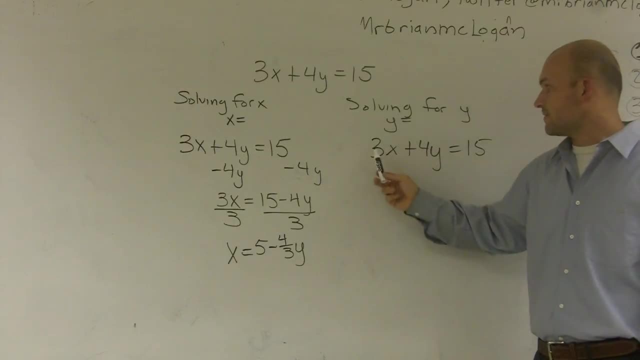 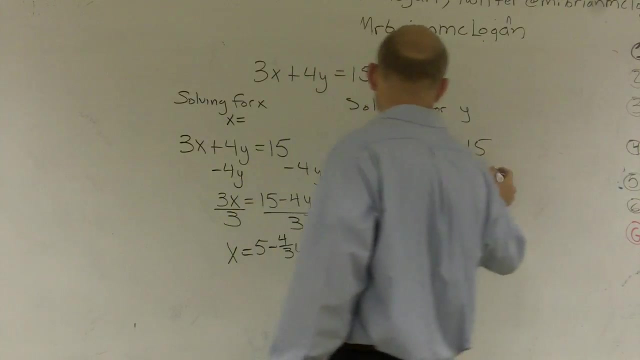 of there. Well, you could write one in but, And I could rearrange this, so we could do it. but just remember, that's a positive 3x. So to get rid of that positive 3x, I need to subtract 3x, So therefore I get: 4y is now equal to 15 minus 3x. Now I need to undo. 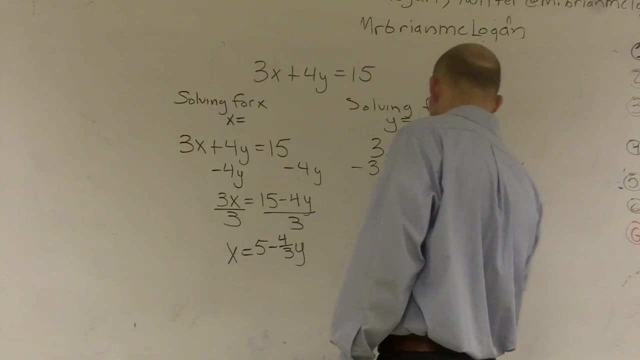 multiplication, by division, And I'll just separate it into two fractions, like that. So that's how you solve for x, That's how you solve for y. There we go.